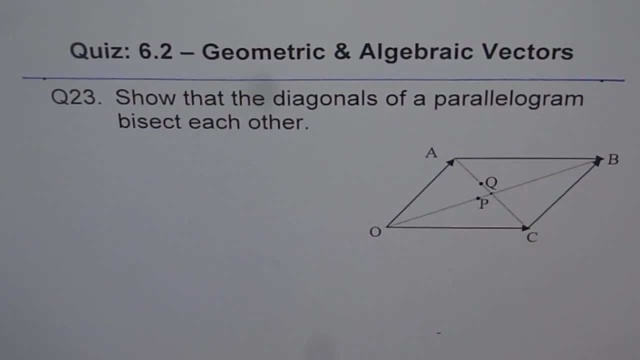 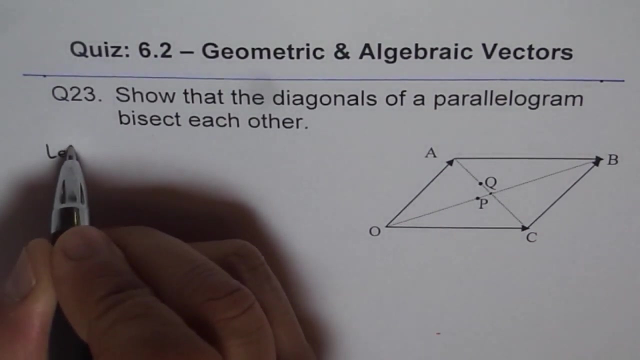 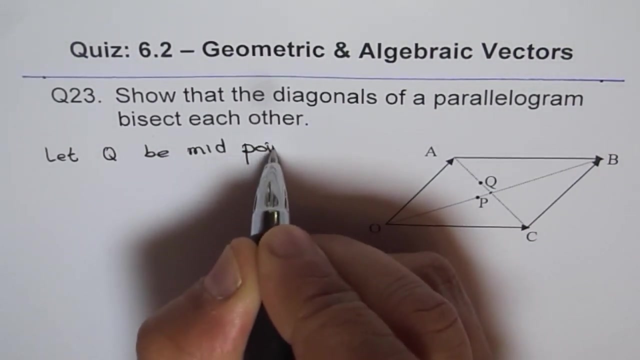 of OB is P. So that means, if the midpoints are different, well they will definitely intersect the diagonals, but we are saying that they don't bisect right. So our assumption here is we are saying: let Q be midpoint of AC. That is what we are. 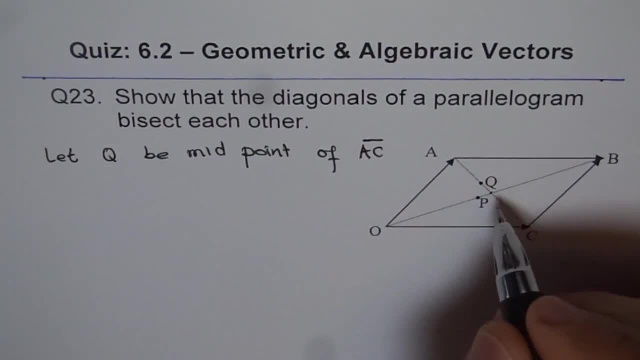 saying That means they are bisecting at a point. and let me call this point as. let me say at present, let's say E, okay, Let's actual point be E, right, And we are saying E is different from the midpoint of the diagonals, That is. 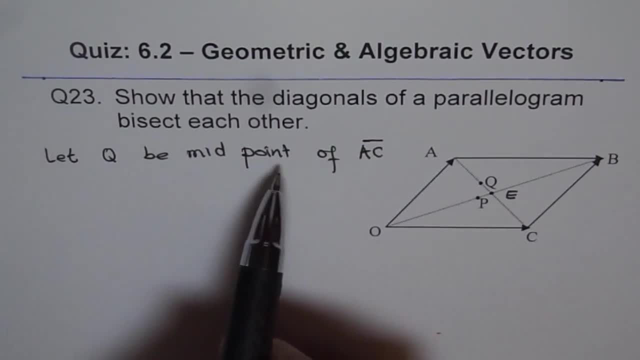 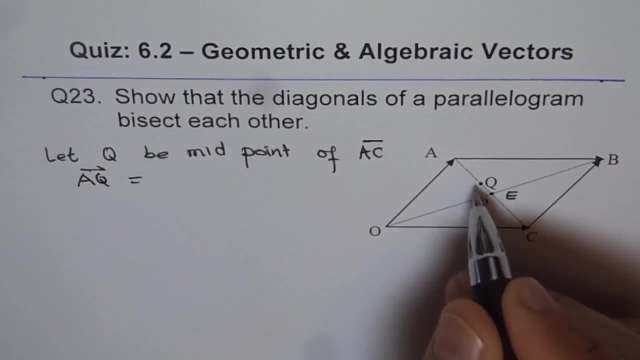 what we are saying right In any case. so let Q be the midpoint of AC. So in that case AQ will be equal to QC, correct After. the direction is same. and when we say Q is the midpoint, then we are saying that Q is the midpoint of AC. So in that case AQ will be. 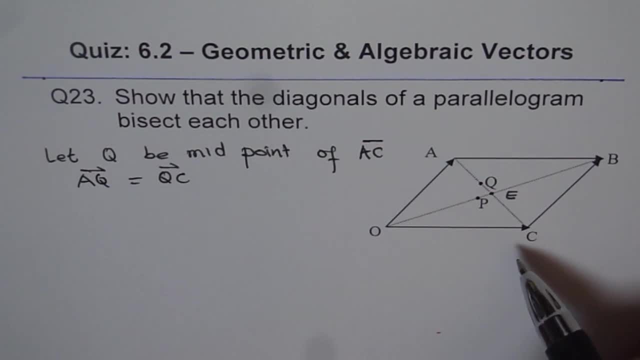 equal to QC. So we are saying their magnitude is also same, correct? So that is what we are trying to say right Now. so that is what we have. Similarly, we will do for the other diagonal also. We will select P be the midpoint of OB, not E, which is the point. 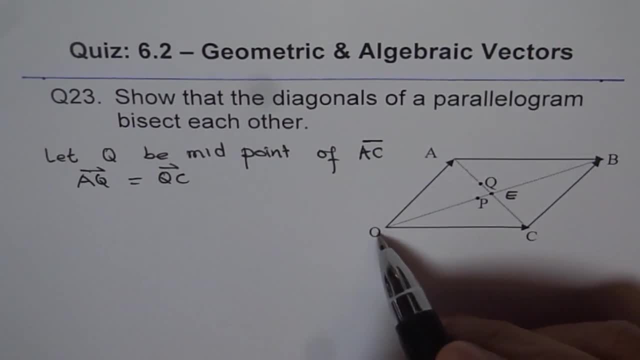 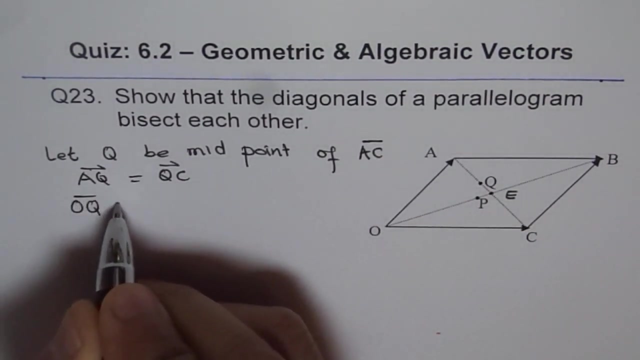 of intersection, And then OP is equal to PB, right? So we are starting by saying that the diagonals don't bisect, And then let's see what happens, right? So that is the kind of approach. Now we say from here, OQ is equal to what We say OQ is equal to. so OQ is equal to. 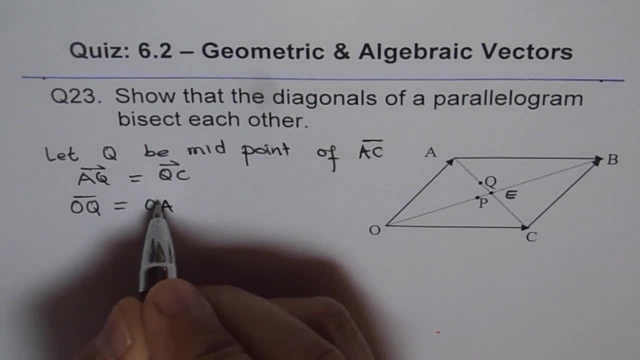 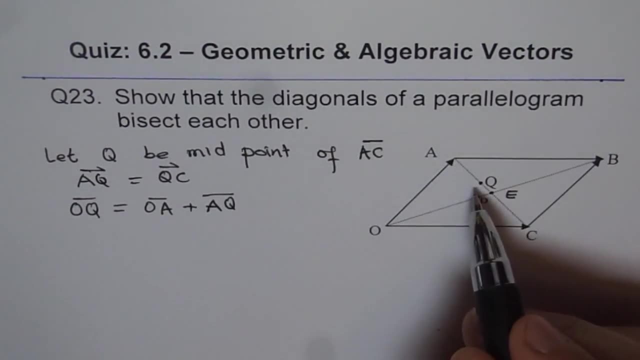 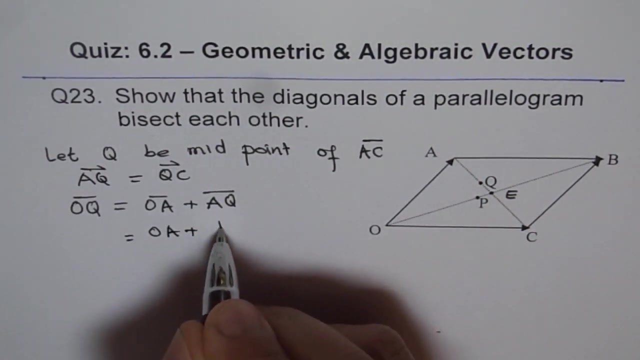 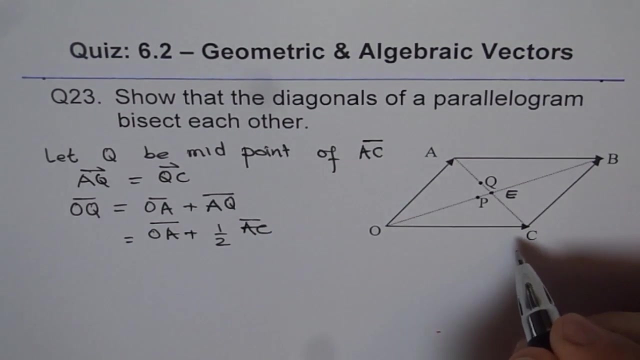 OA plus AQ right. OA plus AQ right. And what is AQ? AQ is half of AC, right. So we could write this as OA plus half of AC. correct, The diagonal AC right, Half of AC. Now, what is AC? I can. 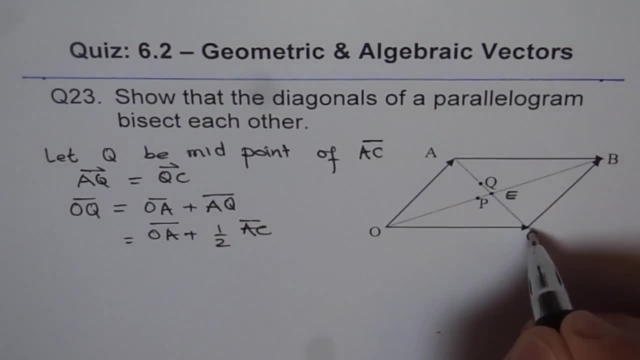 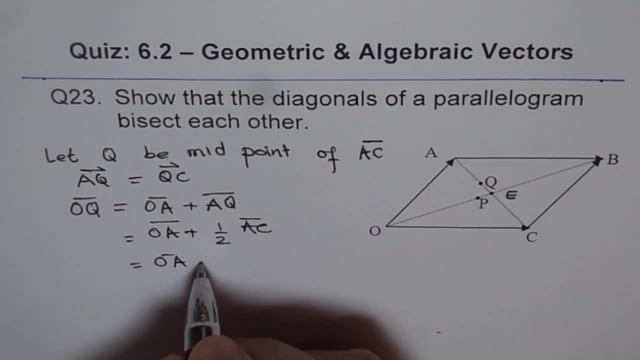 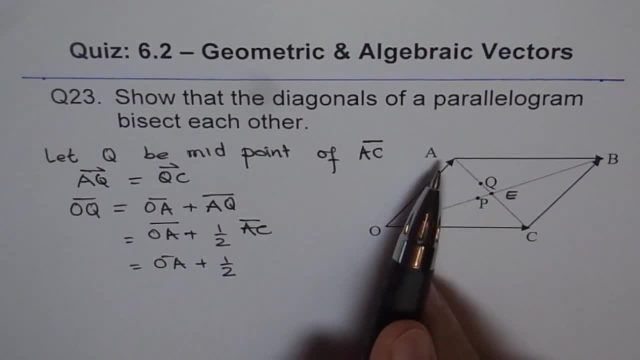 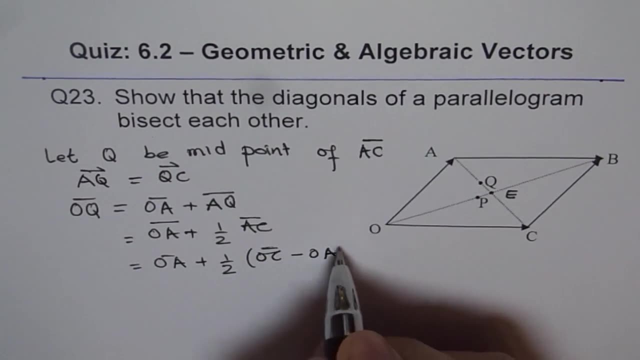 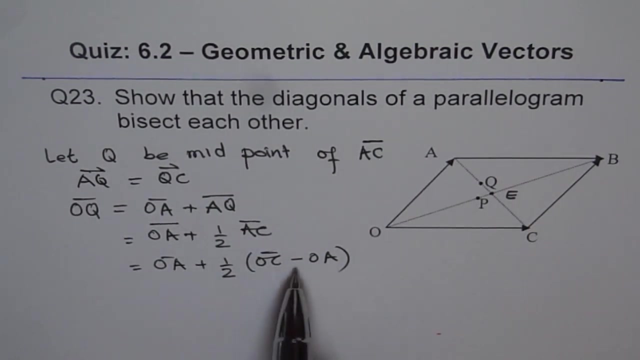 half of AC is like starting from here, ending there right. So OC minus OA correct. So that is how we get this part. Now, if you do your math, OA minus half of OA will give you half OA correct. So I can write this as half of OC plus OA. So OA minus half OA right, OA minus. 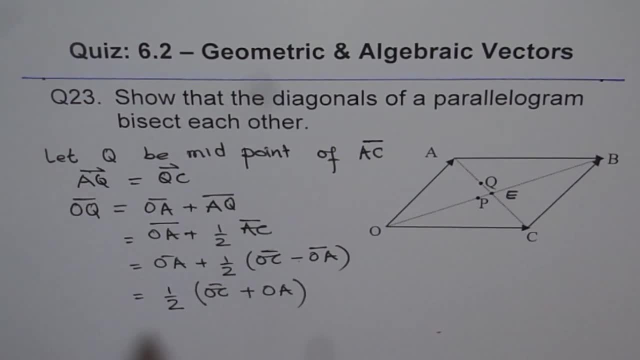 minus half OA gives you plus OA half, So we can get this. So we have proved that O to Q is plus O to A, correct, That's what we have proved. Now let's start with the other side And we'll. 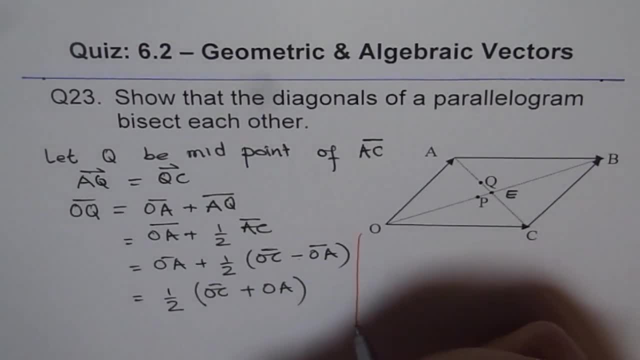 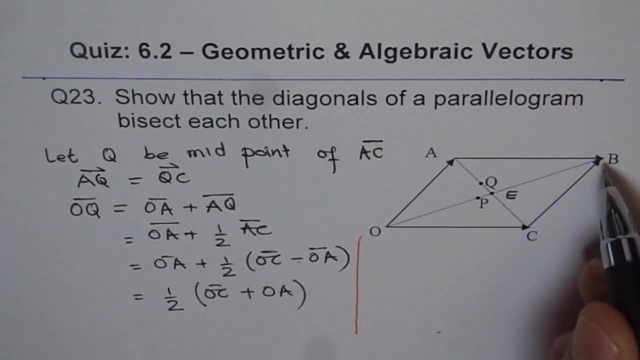 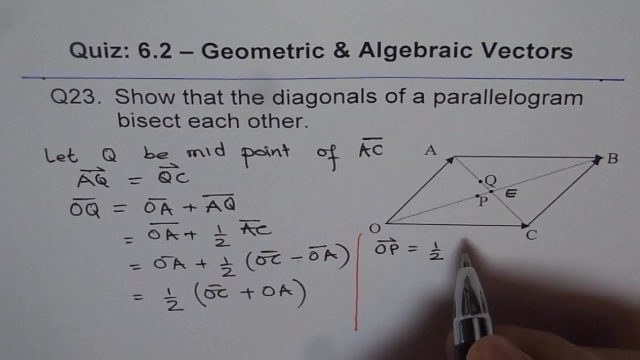 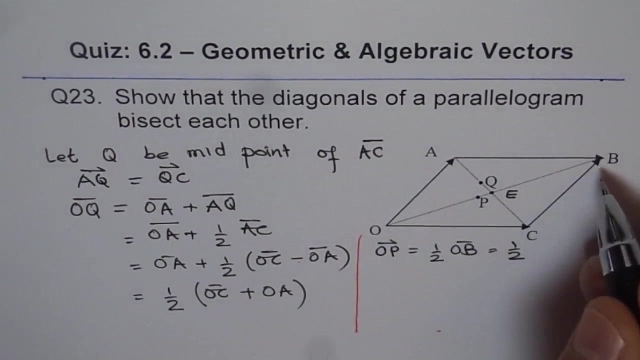 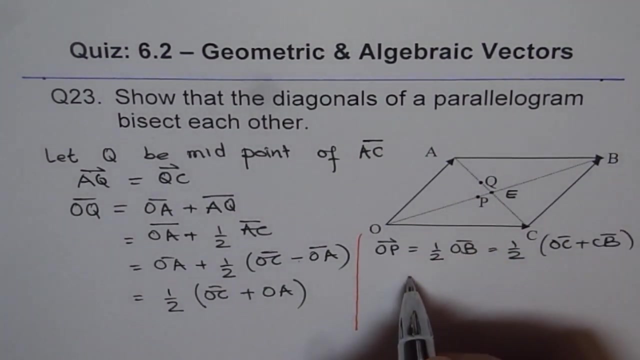 follow the same approach, right. So the approach here is again: let P be the midpoint of OB right. If P is midpoint, then OP is equal to half of the diagonal OB right. Now. that means half OB is equals to OC plus CB. correct OB is OC plus CB right And now. 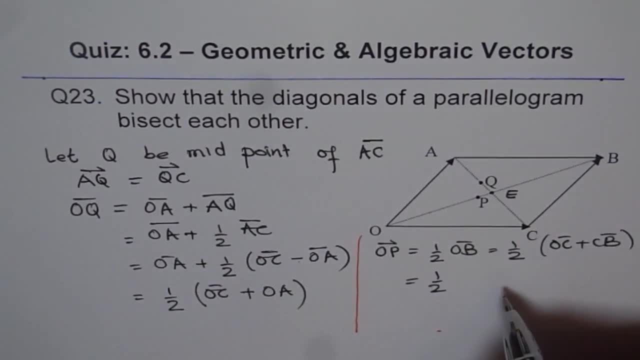 we can write this as half of, so we'll do the same thing, right? So, which is same as half of OC plus OC, Correct? Because CB? we know it's a parallelogram, right? So this side is parallel to OA, correct? 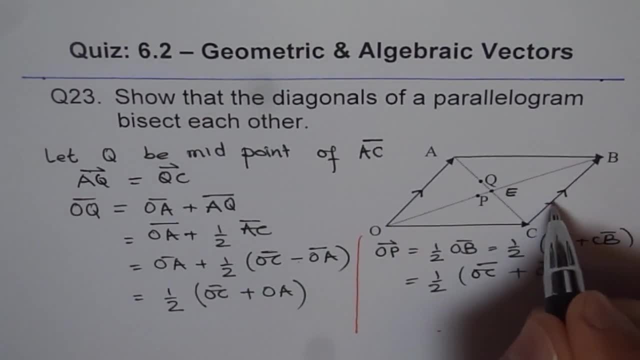 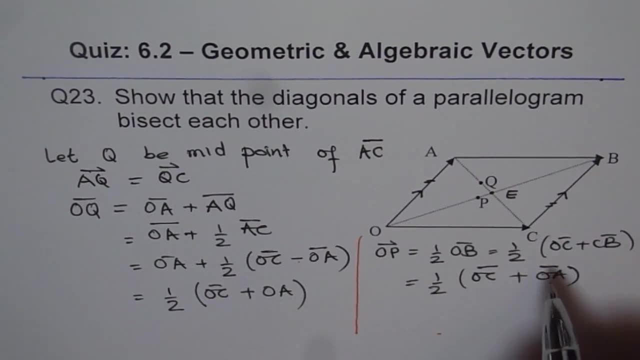 CB is parallel And since it is a parallelogram, these sides are also equal, Isn't that so? And therefore CB is same as OA. So what do we get? We get: OP is same as OQ, Why? Because half of OC plus OA. let me get back to the first equation. So this is our first equation.